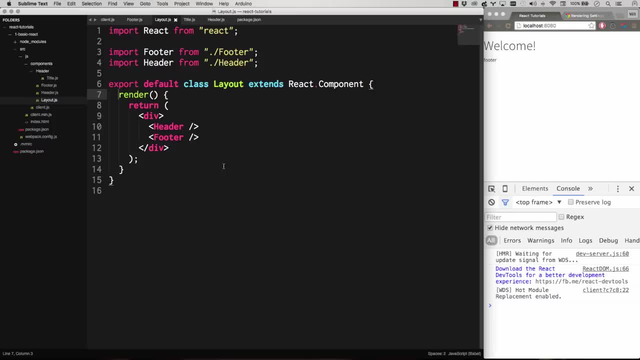 third way context, but it's a little bit more of an advanced feature and the API is not guaranteed stabilized, as it's something newer to React, So we're going to leave that out for now. We'll touch it a little bit more later on in the course. So let's look at state first and as you go you'll end. 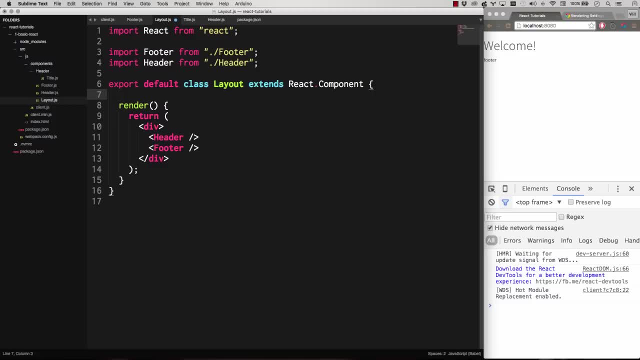 up using props much, much more. but state is also used by a lot of people in some ways as well. So state is basically available through this dot state, which by default is null. So by default state will be null And then you can set it. So let's go. 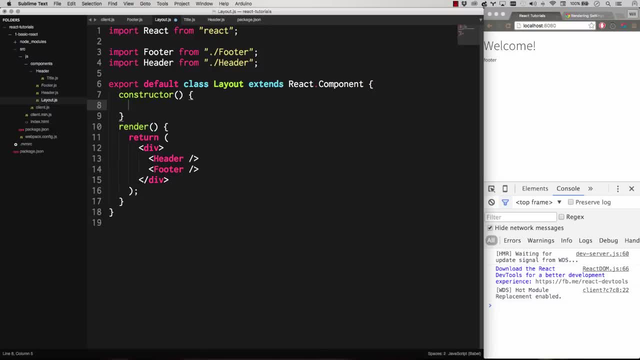 ahead and make a constructor method, and the only place you want to set state way is in the constructor method. you literally just set your initial state. this state equals name, will, and then we can access this by entering this dot name, states, dot name. so you see, it's kind of a similar concept to what I did. 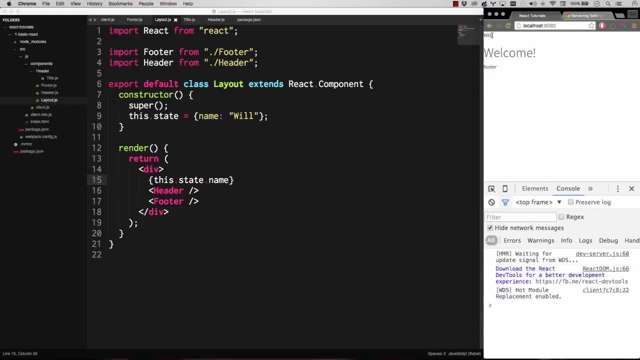 earlier, but this is the proper way to do it. so you see that. there you go. my name will is printed on top. now what's really cool about state is whenever state changes on a component, the component will automatically rerender and update the Dom if there are any changes. if there are no changes, the Dom won't get. 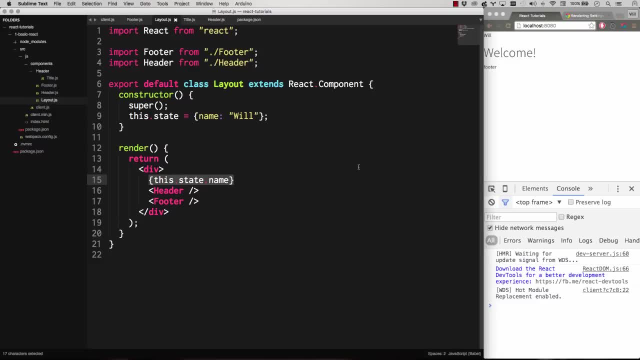 touched at all. that's the first big amazing thing that react brought to the world is it manages a virtual Dom for you. so whenever react renders out all the components- the component tree is what it's called- it renders the layout, the header, the footer, everything. then it looks for changes from the virtual Dom. 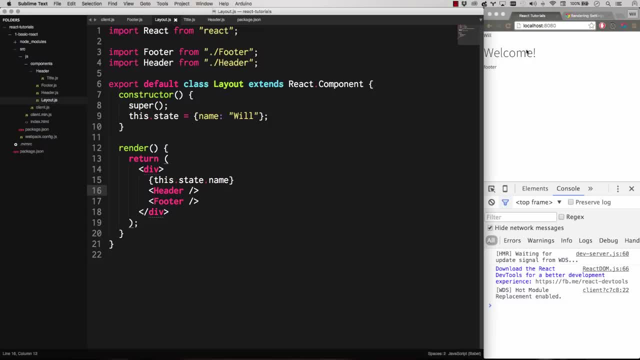 to the actual component and then it looks for changes to the actual component. if there are changes, it will update only the affected nodes in the most efficient way. if there's no changes at all, it doesn't even touch the web page. this is great, because JavaScript is really really fast, but the Dom is really. 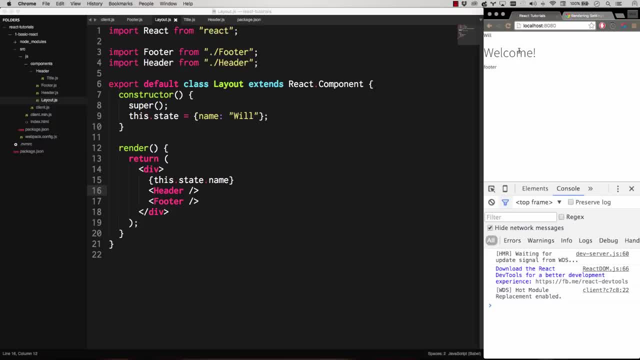 really slow whenever we have to actually go to the DOM and update elements. that's the slow part of any webpage. so by having a virtual Dom where everything is updated behind the scenes and only changed in the real Dom if there's differences, that allows our applications to become extremely fast. 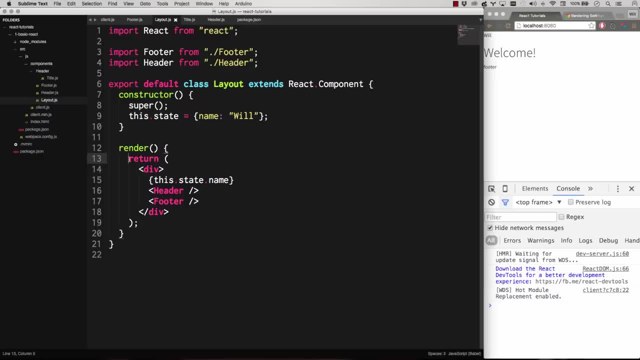 So let's go ahead and look at how we change the state. We could go ahead in this render method, do a setTimeout. Let's pretend after one second the user did some action and we wanna change our state, So we're gonna go this setState. 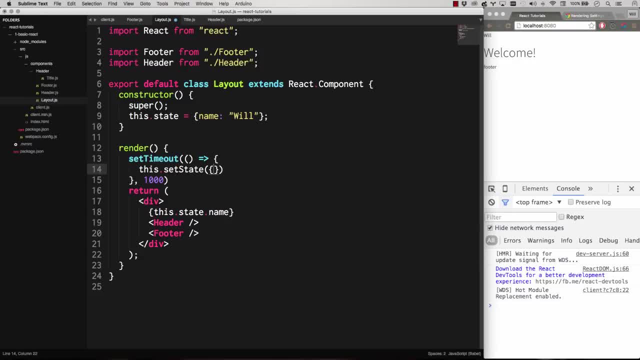 That's the one method that you need to know with state, And you just give it a new state. In this case, our name is now changed to Bob, And so when setState gets fired it will update the state and then that will automatically re-render. 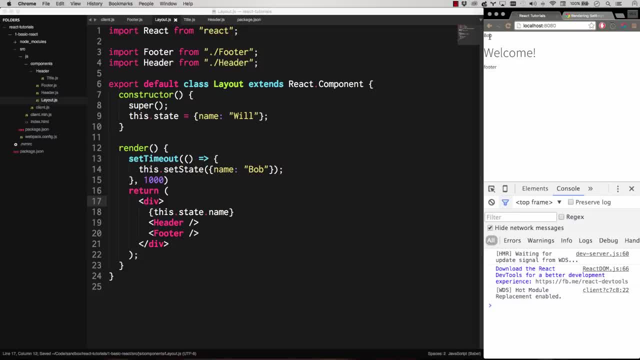 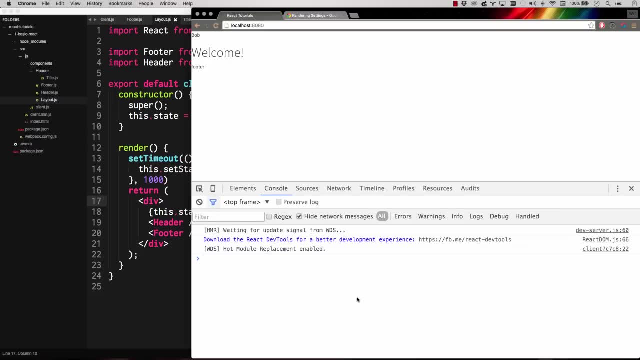 And again, if there's any changes, it will print out. You see, it went from Will to Bob. Let's actually show you what React is doing behind the scenes. In my console on Chrome, I'm gonna hit the escape key And that gives me these rendering options. 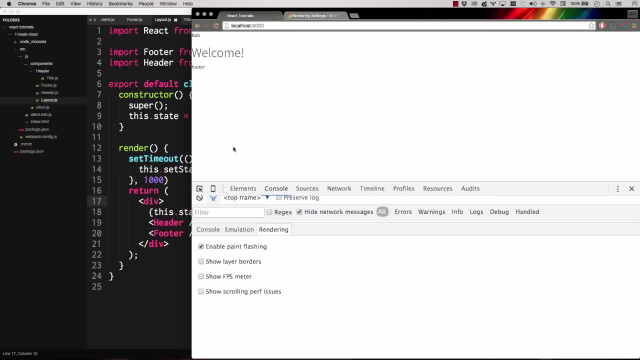 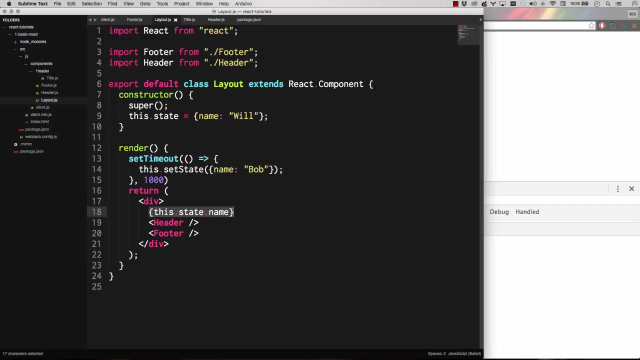 I can enable paint flashing, So now the screen will flash green whenever a node gets changed. You can see: first the whole screen was green and one second later Bob changed Only Bob, nothing else, Even though we did a complete new render of the header, the footer, the entire layout. 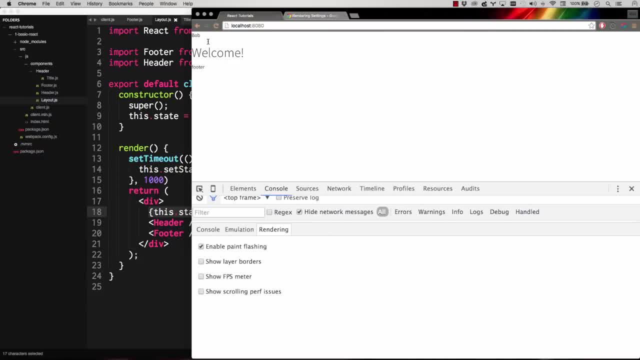 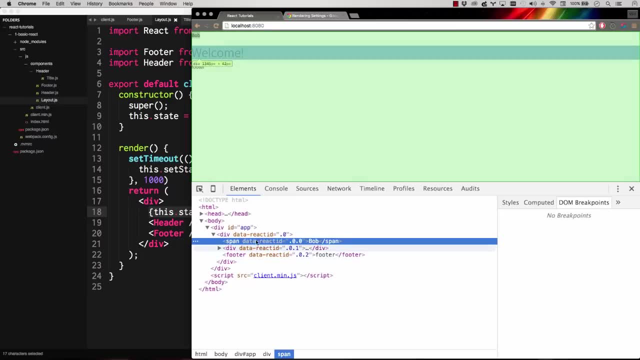 the only actual DOM element that changed was the one that contains state name. So that's all that React updated. I'm gonna go ahead and update this here or inspect this, And you can see that it automatically made a span for Bob. That's the only thing that will change. 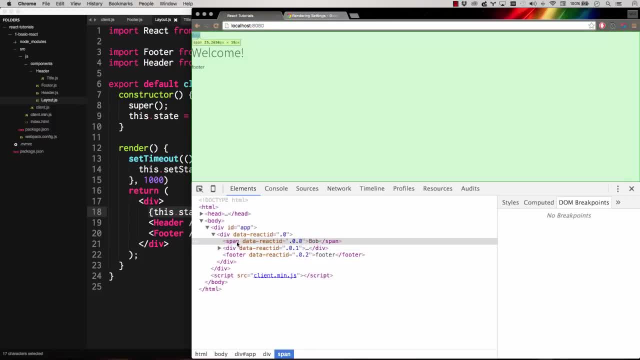 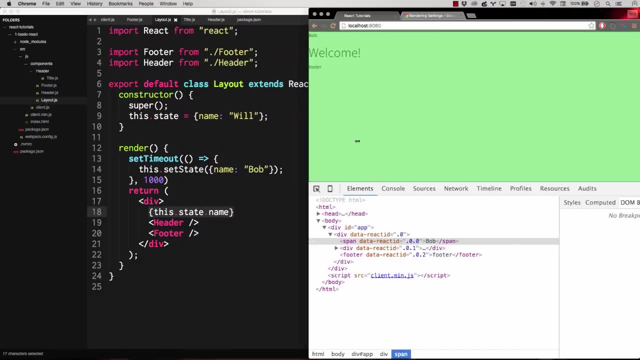 Let's go to refresh again. Flash is green And the only thing that flashed changed was this span for Bob: Excellent. So React automatically manages the DOM manipulation for us. This is one of the best things, in my opinion, to React Cause if you've done Backbone at all. 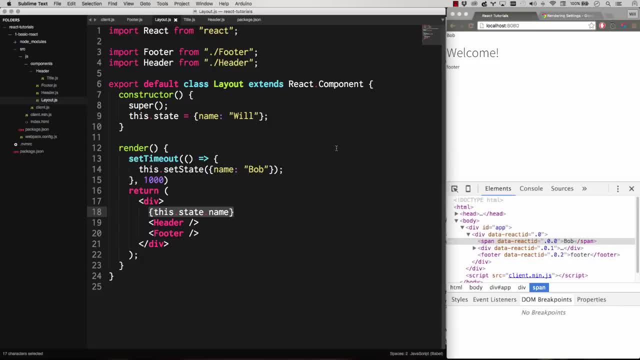 you understand that there's always this question of: hmm, at what point should I update the DOM And when I do, who should update that? Should the list component update the whole list and re-render the whole list, Or should just each list item manage the DOM? 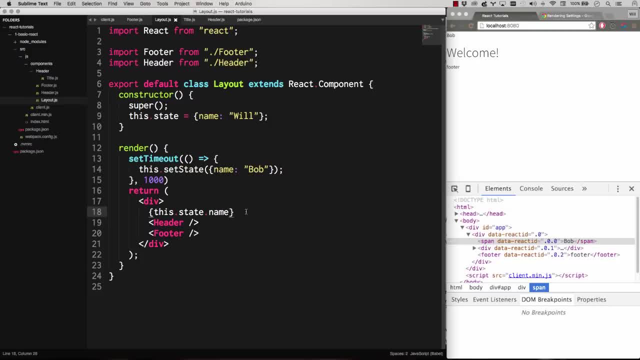 Or should the list component update the whole list? And the answer to that is: if you've done Backbone at all, you're gonna have to re-render the whole list, And if you've done Backbone at all, you're gonna have to re-render the whole list. 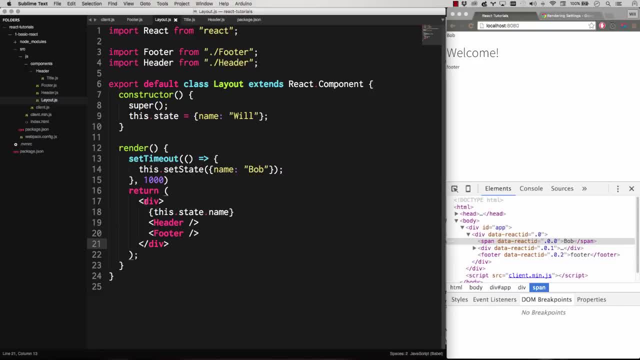 And if you've done Backbone at all, you're gonna have to re-render the whole list And basically React takes all of that out and says: we're gonna re-render everything all the time on any change, but we're only gonna do it in JavaScript. 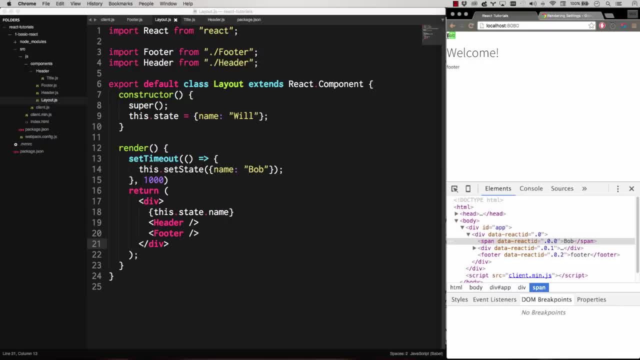 and we're only gonna touch the DOM if something is actually changed. that would reflect in a visual way. So that's the great first thing about React. I hope that made sense And that's how you'd manage. state: The header could have its own state as well. 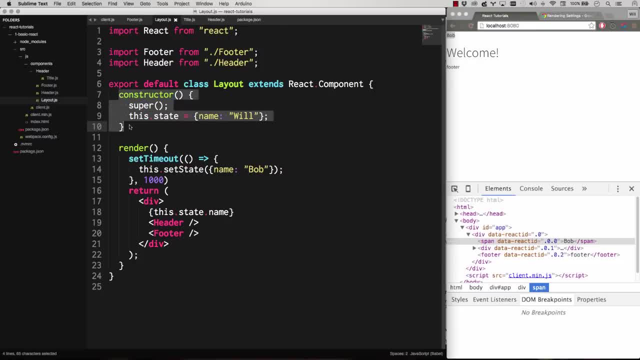 So kind of the mentality behind state is state only gets used if a component has an internal value that only affects that component and doesn't affect any of the rest of the app. If there's something that affects layout and affects absolutely nothing else, state may be appropriate. 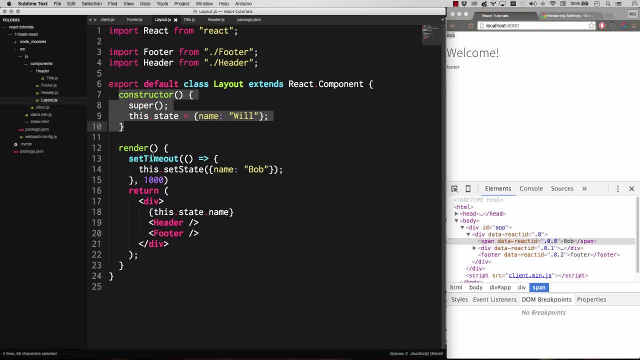 Aside from that, you wanna use props, And props are injected into every other component. Let me show you how props work. Let's get rid of all this state, get rid of the state name, and we're going to now inject a prop into header. 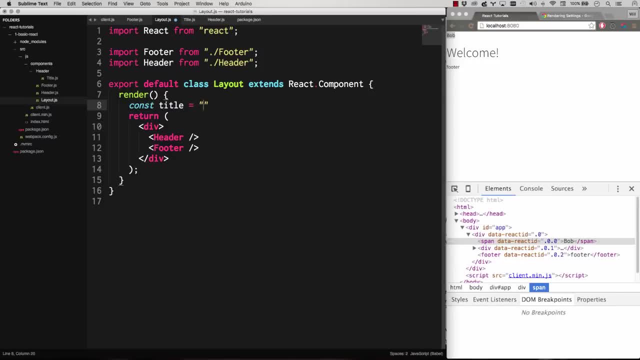 Let's say var title. we'll do a const. Title equals welcome will. And now my header. I'm actually going to inject a title: Title equals title. There we go. So I've basically created a prop, just like you would on an actual DOM element. 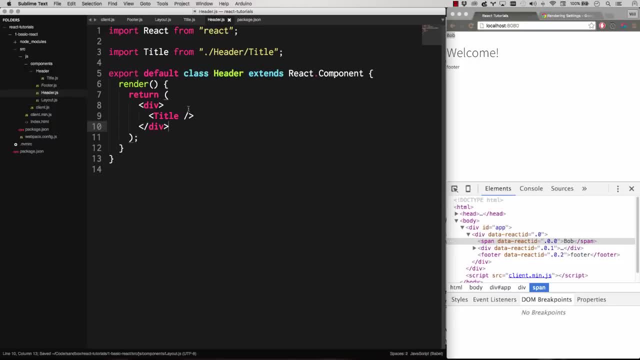 You'd give it a prop. So now if I go to my headerjs I can access thisprops. Let's do a console log of thisprops and see what we're getting here. Let's look at my console. You can see that I have a title of welcome will. 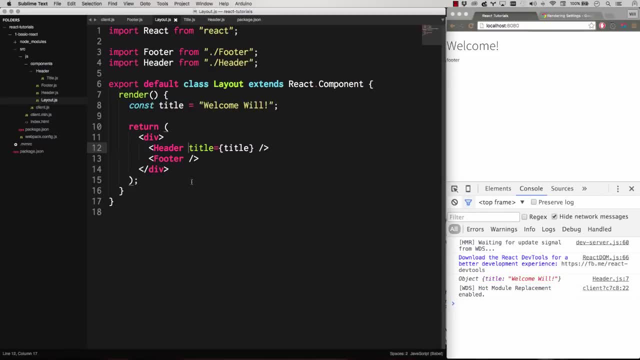 So it automatically gets converted into an object. I could give this multiple props. I could give it a. let's see, name equals something. We'll just give it a brand new string right there. You can see that I have. name is something. 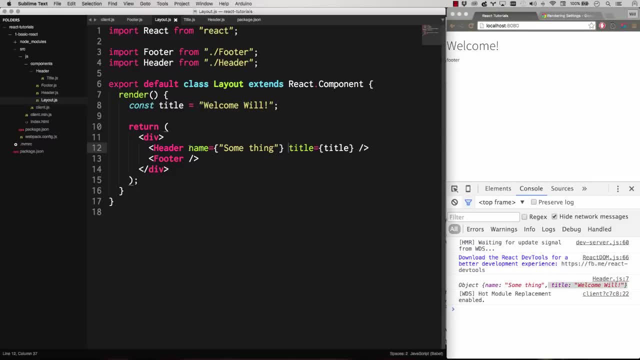 and title is welcome will. So that's how you inject props into things. I could create a second header and I could give its title something else, And again, that's how we're going to actually create multiple versions of a header that are different. 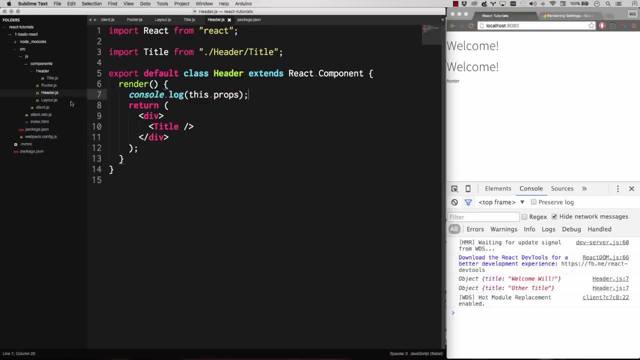 So let's make that header now use a different title. So in header we're going to actually just continue props. right on over to title We're going to go: title equals thisprops title. So we're just going to continue passing that straight. 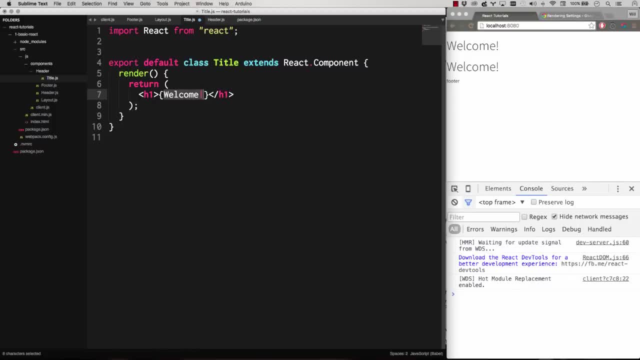 on through to title and title will actually make use of it. There we go. So now we have welcome will and we have other title They've rendered through. Our layout has passed in a different title to each header. Our header is just transparently passing them through. 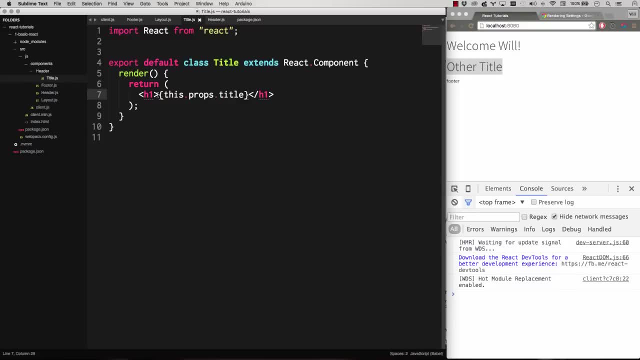 to the title, only the title prop, And then our title is actually receiving that and spitting it out. So we have a completely different header and we have a completely different footer for each one. And again, let's go ahead and look at this. 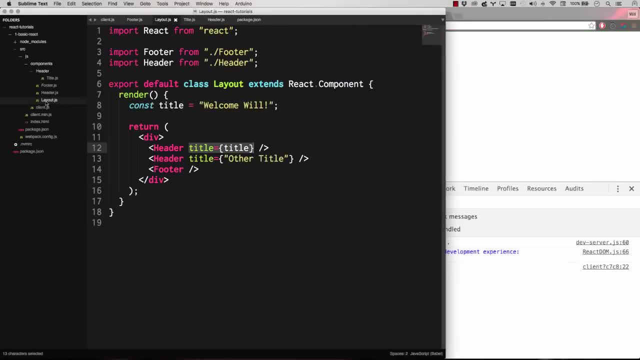 And now what I can do is I could let's go ahead and change our layout here to use both state and title. Now let's do our super. this state equals title, So by default our title will be welcome, And let's go ahead and pass in this dot state, dot title. 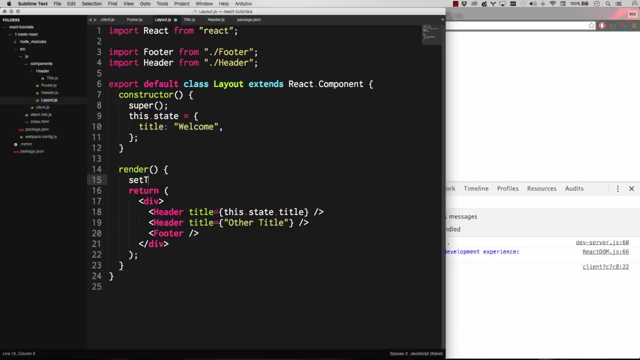 And we'll leave that one there as well. So then again our setTimeout. let's make this two seconds. I felt like one was a little too fast to catch. We're going to change our state, So basically changing it from title to title. 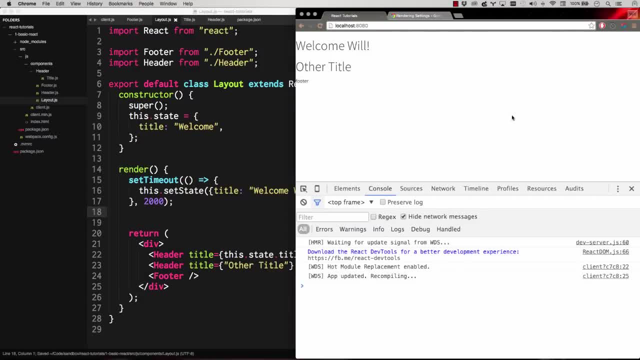 because we had already gone through it from welcome to welcome will. Let's go and see what happens over here. You can see that after two seconds our header component got updated. Let's go ahead back to these elements and let's see if the header or the header and the title got updated. So this is our header component. 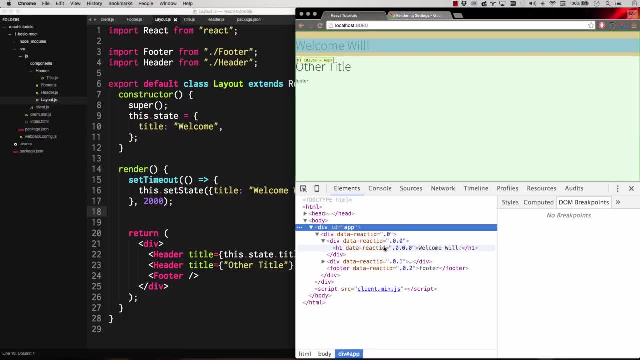 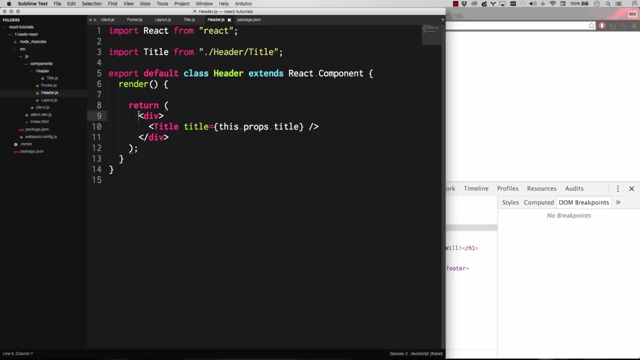 This is our title component. header component- title component. Let's refresh. You can see that two seconds in. only the H1 changed. That's because, even though our header component received an update, our header component received a new prop. it rendered out the exact. 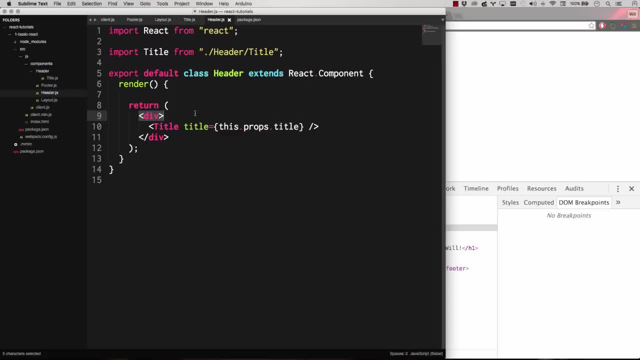 same div, no changes. So it didn't re-render this div to the DOM. Then it re-rendered a child component of title. That changed. The DOM looks different for the H1 that it renders. So it updated the H1 and the H1 only Again. once you get this concept, it's really monumentally huge. 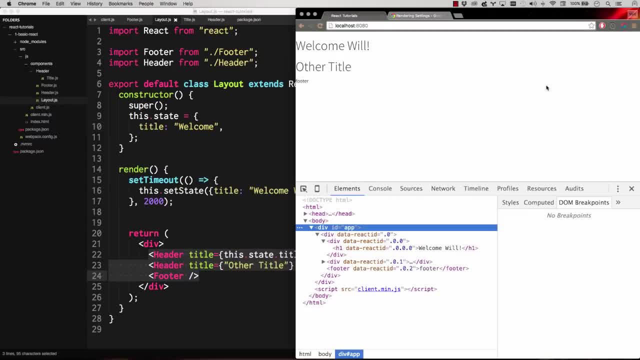 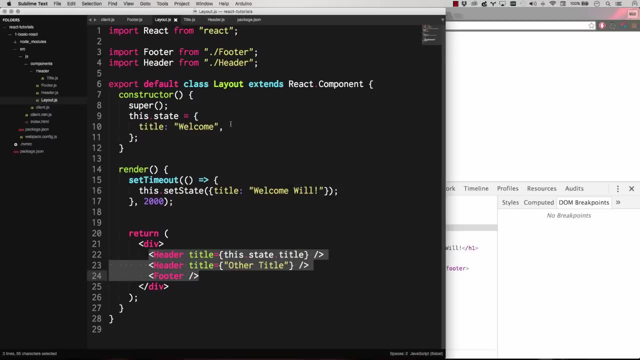 No matter how many components change. we're only going to update the DOM with the H1. The actual element changes that got created when the entire tree rendered. So there you go. That's the basics on how we manage data within our components. Let's go.